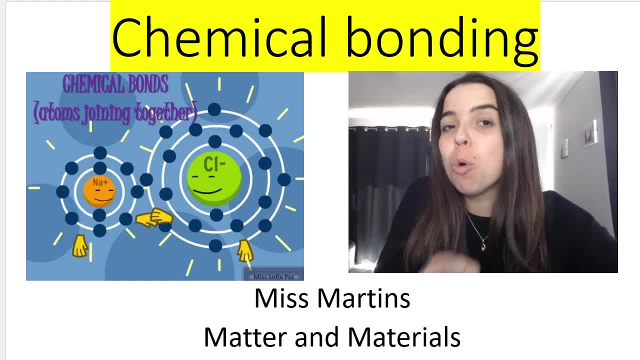 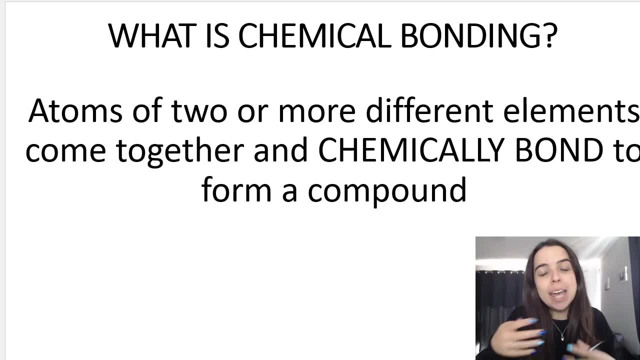 and don't forget to give this one a thumbs up and subscribe for more maths and science videos. So what is chemical bonding and why does it happen? When chemical bonding occurs, a chemical change takes place. We have atoms of certain elements, different elements, coming together, and when 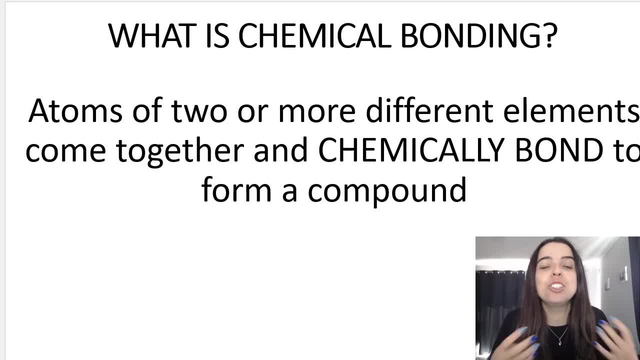 they chemically bond. when that chemical process, that chemical change happens, they form a new product with different properties relative to the starting reactants. So what I mean, for example, is we can have hydrogen, which is a gas, H2, hydrogen gas plus oxygen. Those can bond to form H2,. 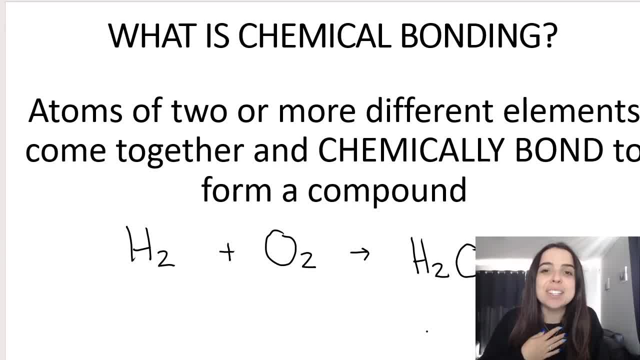 O, water which we drink, which we need in order to survive, Right? so that is basically chemical bonding, and here you'll see. the definition says: atoms of two or more different elements come together and chemically bond to form a compound, So H2O or water, for example. let's think of another. 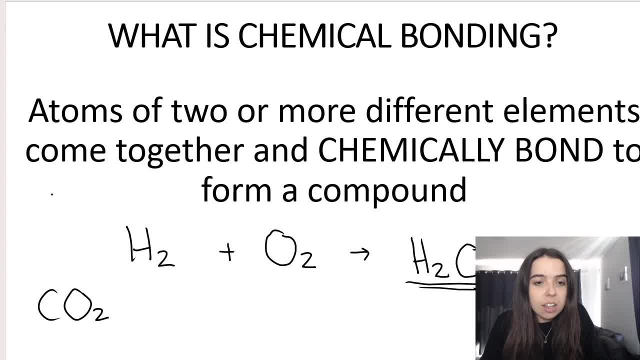 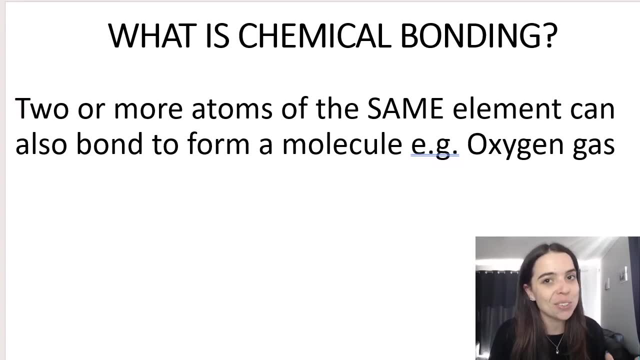 one carbon dioxide, that is a compound, sulfur dioxide, maybe potassium nitrate. These are all compounds, these are atoms, or of two or more different elements, and when they bond they form a compound. Now, this is slightly different to what we call a molecule, just slightly different. 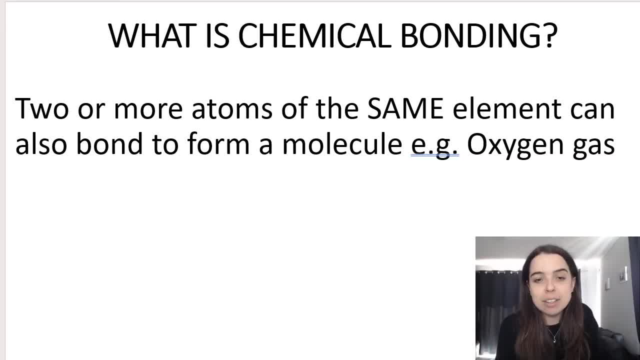 terminology When two or more atoms of the same element when they bond, they can form a molecule. I'm sure you've heard of diatomic molecules such as oxygen gas. Now here's a little rhyme. have no fear of ice cold, I don't know, beer, I guess. So H2 is high in oxygen, G2 is high in hydrogen. 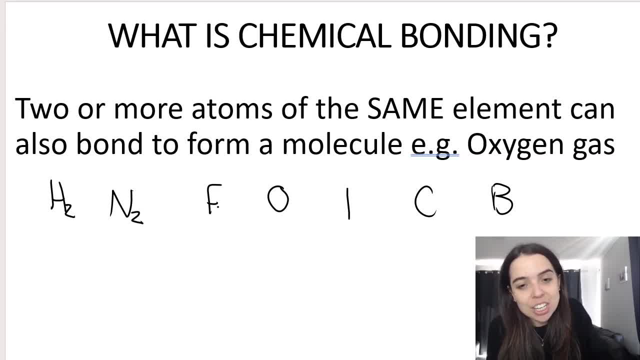 I don't know, beer, I guess. So H2 is high in carbon. so H2 is high in carbon, I don't know. So H2 is high in oxygen hydrogen. N2 is nitrogen, fluorine, oxygen, iodine. this is chlorine and bromine. These are two or. 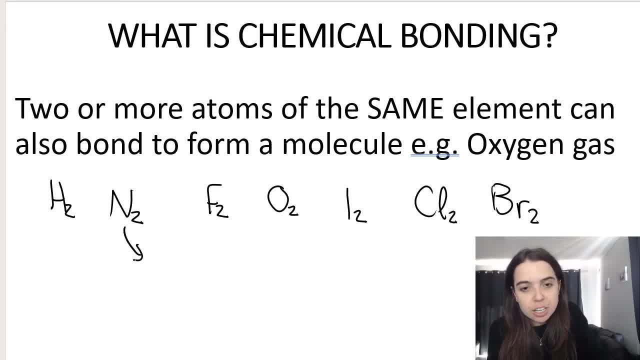 more atoms of the same element. So, for example, nitrogen is a nitrogen atom and a nitrogen atom. two or more atoms from the same element- okay, They form a molecule. just remember that. Now, if we look at how bonding happens, it can take place in many different ways. but before we get there, 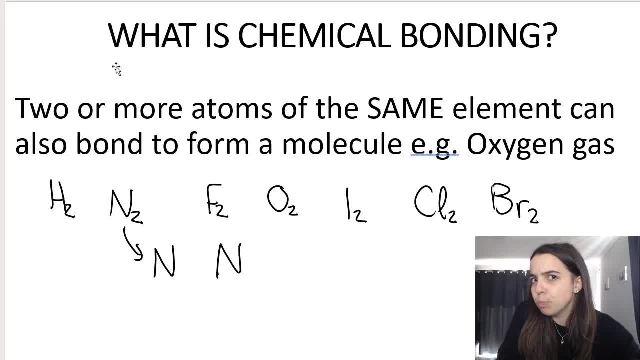 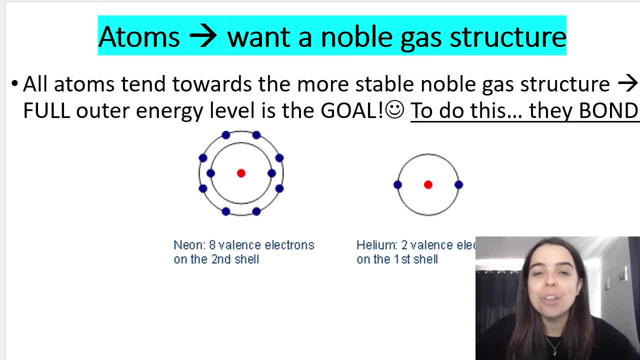 why does bonding happen? What is the purpose? Why bond? Essentially, atoms want a noble gas structure, they want to be stable, they want full orbitals, full outer energy levels. that's the goal. They tend towards the more stable noble gas structures. and the way that they achieve this. 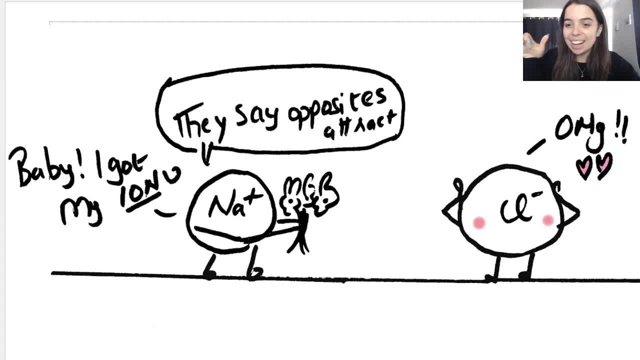 goal is that they bond. Now I thought that this is really, really cute. see if you can look at this and make sense of it. This over here is Na+, that is a sodium ion. it's a positive ion, a cation, and this is Cl- it's a. 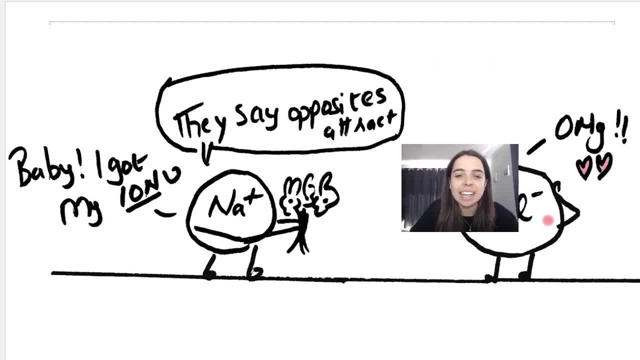 chloride ion, an anion, a negative ion, and you'll see what it says over here. the little sodium ion is saying: baby, I got my ion, you ion, and they say opposites attract. So this is a little example. 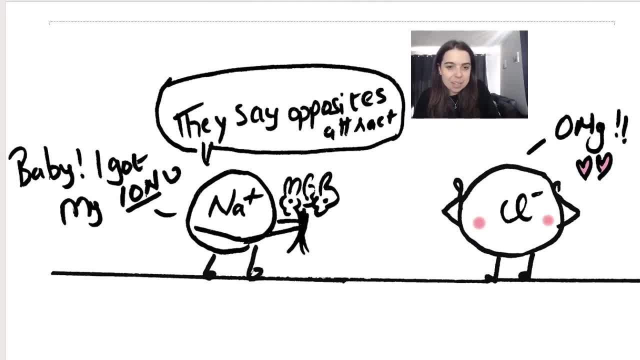 of ionic bonding. See here it says my ion ion. Now remember we spoke about cations. cations are positive, they're positive, ions positive and anions: onions are negative, they make you cry. anions and these are. 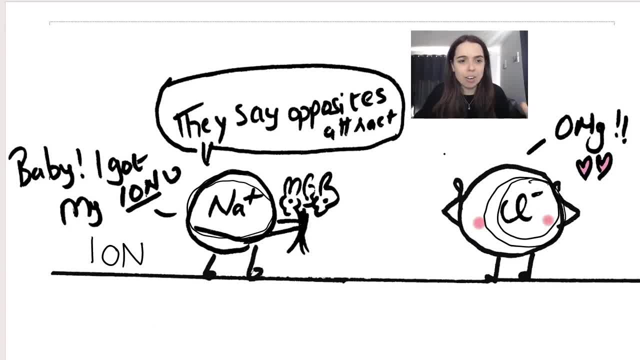 opposites. so then they attract and they bond. because of this, This is ionic. but there's another type of bonding that you need to know and you need to be familiar with, and that's called covalent bonding. Let's have a quick look at the difference in terms of how we draw the Lewis dot diagrams. 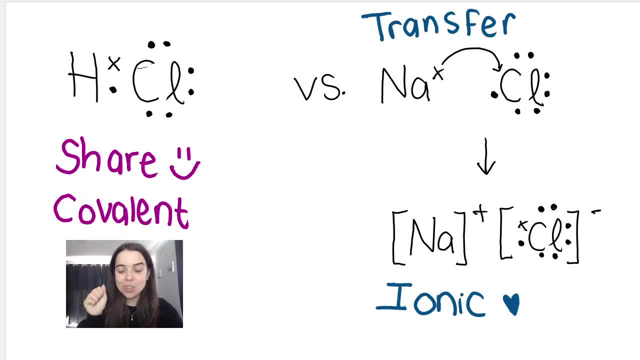 Now what you see on the screen. I don't want you to panic. these are Lewis dot diagrams. these basically visual representations of two atoms when they bond, but you can see the difference Above me over here. this represents a covalent bond. Now this involves the sharing of electrons. 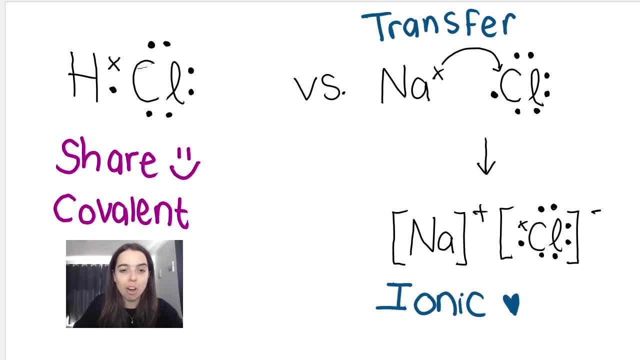 between two or more atoms to form a molecule or a compound. So over here you can see that the hydrogen and the chlorine are sharing electrons Here. so this was the example of the picture that I just showed you. This is an example of an ionic bond. 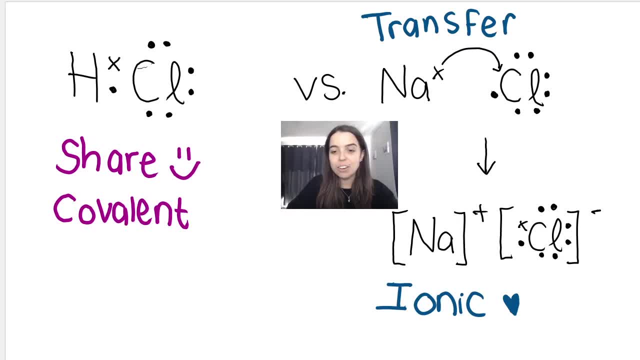 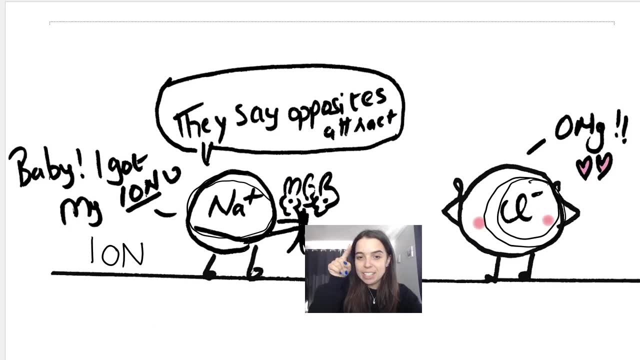 which involves the transfer of electrons. If we look at that little picture again, we can see that the sodium ion over here is giving something to the chloride ion. Basically what happens is the sodium ion gives the chloride ion an electron. You can see here the sodium ion has an extra electron. 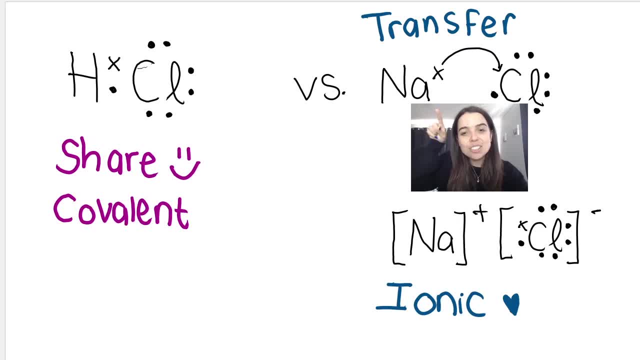 The reason why will become clear. Soon gives an electron to the chloride ion and that transfer of electrons causes our sodium ion to get a positive charge, a chloride ion to get a negative charge, and then they attract, they bond. This is ionic. 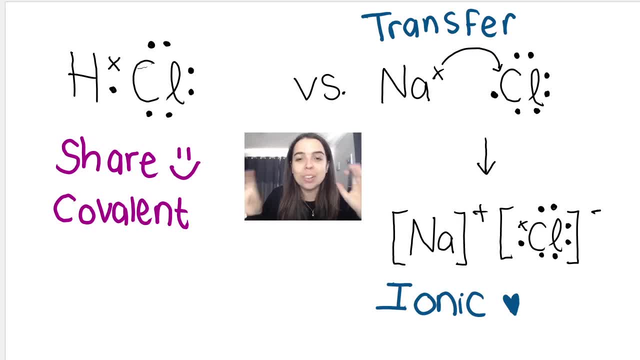 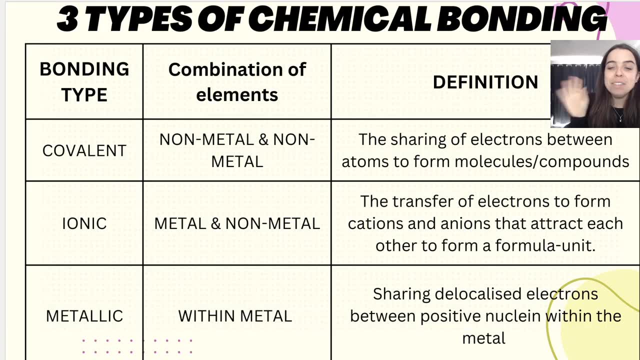 Now these Lewis dot diagrams and how to draw them. we will cover that in the next video. but it's very important to notice the difference and to understand the difference. So I've summarized the three types of chemical bonding or intramolecular forces. 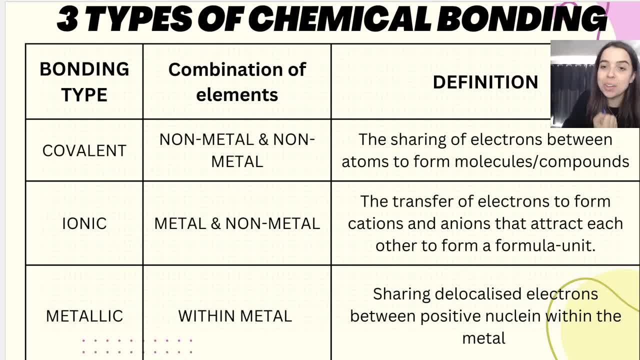 intramolecular forces and intramolecular forces. Intramolecular means within the molecule, Intra is within, So bonds are within or inside the molecule. These are the three types that we will be going over. Covalent is the sharing of electrons like I. 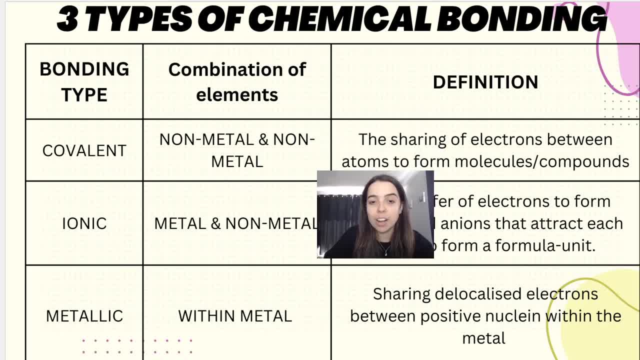 showed you in the previous slide. And then we've got ionic, which is the transfer of electrons, So electron given from a metal to a non-metal, the transfer, that's ionic And then metallic and that is essentially within the metal. 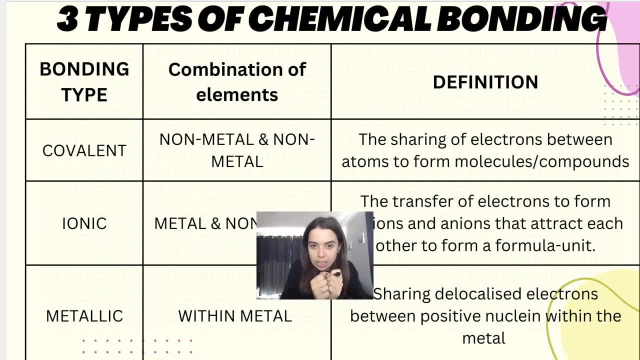 It's when metal positive nuclei, the atoms of the metal they share electrons, delocalize electrons. I will show you that in a future video, But for now we're going to focus on these top two, which is you need to be able to draw the Lewis dot. 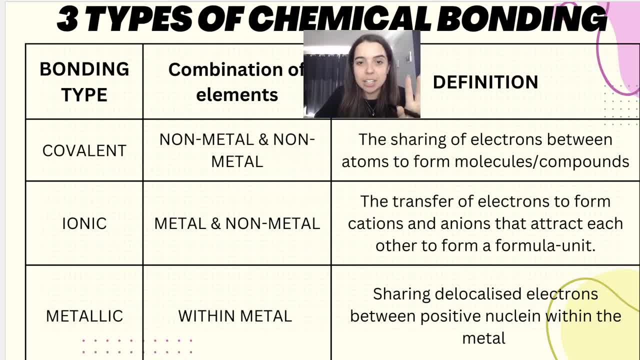 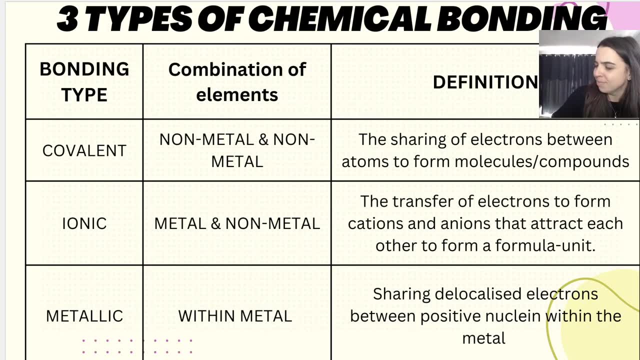 diagrams for these. Another very important thing is that you need to know that covalent bonding takes place between a non-metal and a non-metal. Ionic bonding is between a metal and a non-metal. Okay, now you might be thinking I forgot how to tell the difference. How do I know? 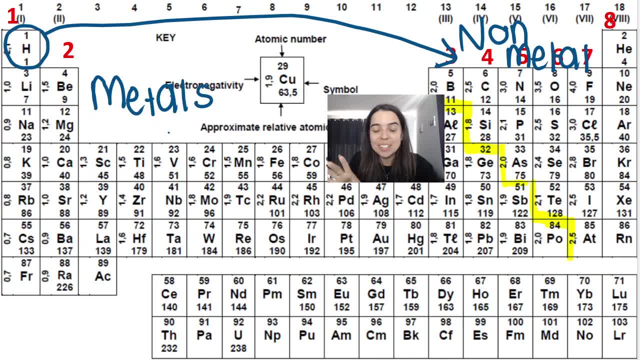 which are metal and which are non-metal. If we look at the periodic table over here, on the left hand side we have our metals, except for hydrogen. So you see I've circled hydrogen. Hydrogen is not a metal. So metals are on the left hand side. non-metals, as well as hydrogen, are on the right. 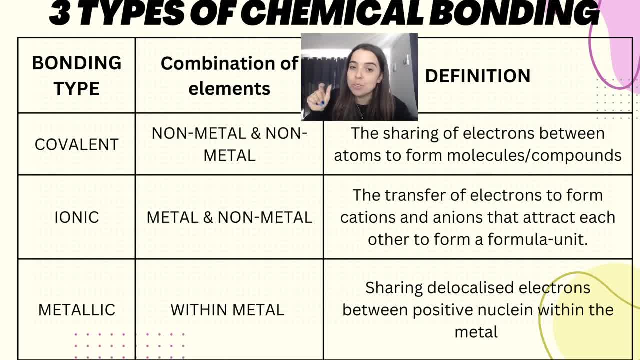 hand side over there Right. so now we know if we have two non-metals, so for example a hydrogen, and we have a chlorine, that is a covalent bond, H2O, again covalent bond. they share electrons. 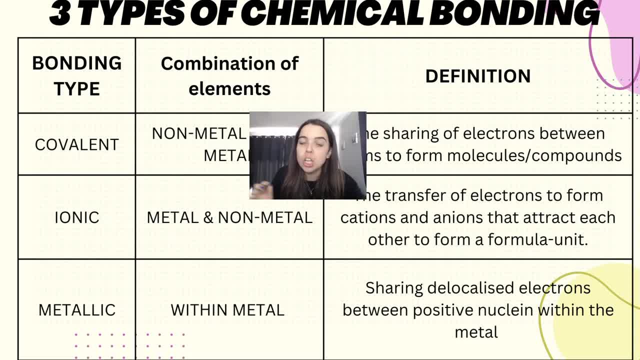 Ionic would be between a metal on the one side of the periodic table, non-metal on the other side. So for example, magnesium and fluorine. We'll get to metallic later. The last thing that's very important to know before we get into Lewis dot diagrams is that 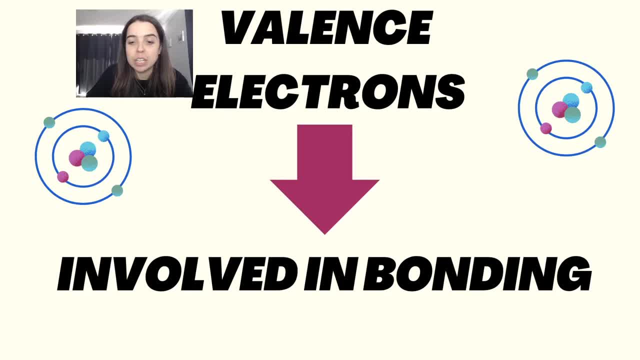 it is our valence electrons that are involved in bonding, And you should remember that valence electrons, those are the electrons in the outer orbitals, So the outer energy levels. those are our valence electrons, The electrons on the outside. Now, how do we know very quickly what? 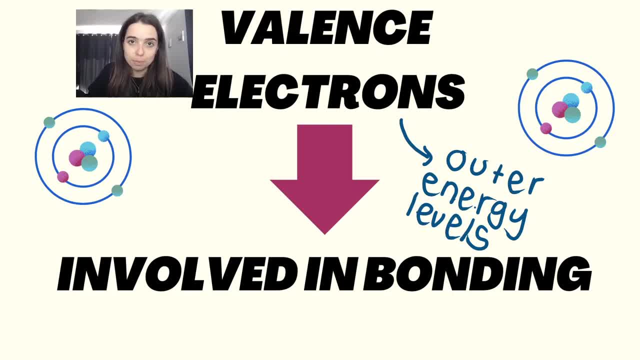 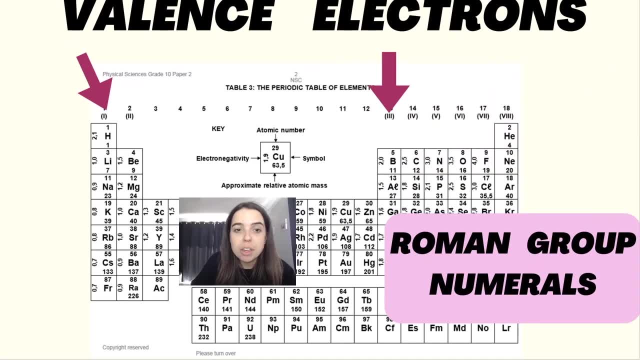 our number of valence electrons are for each of our different atoms. Well, if we look at our periodic table we can see the Roman group numerals. So you can see here on the top of every group we have Roman numerals. So that's number one. then we've 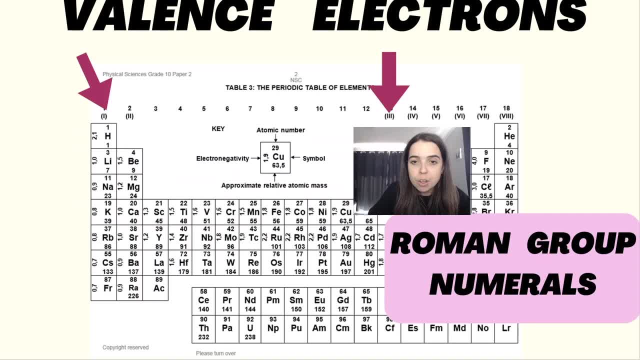 got two, then we skip this middle part. we have three, four, five and so on. Those Roman group numerals indicate the number of valence electrons. So, for example, if I ask you how many valence electrons oxygen has, you'll look at the Roman group numeral and you'll tell me that oxygen has. 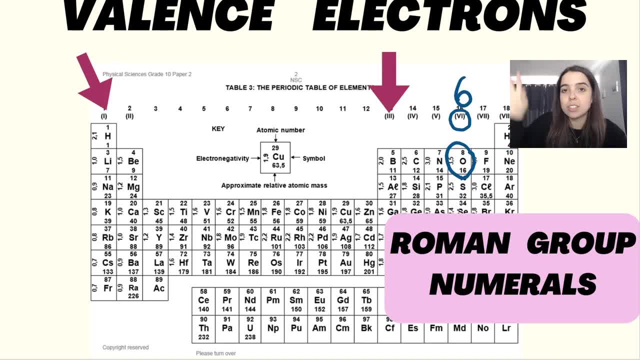 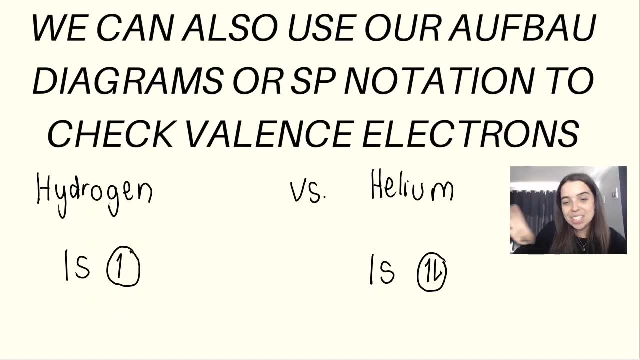 six valence electrons, which means six electrons in its outer energy level. The reason why this is important is it's because it's these electrons, the valence electrons, that are shared if it's a covalent bond, or transferred if it's an ionic bond. This is, if you want to be. 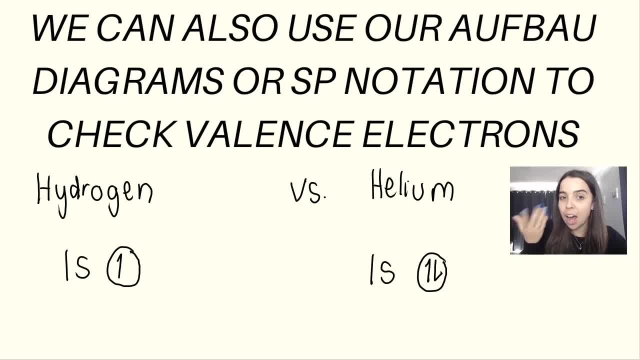 really fancy and really know that. you understand. We can also use Aufbau diagrams, which is what you see over here, or SP notations to check valence electrons. If you don't know how to draw Aufbau diagrams or do SP notations, you're going to want to watch my video on that, which I will link for.